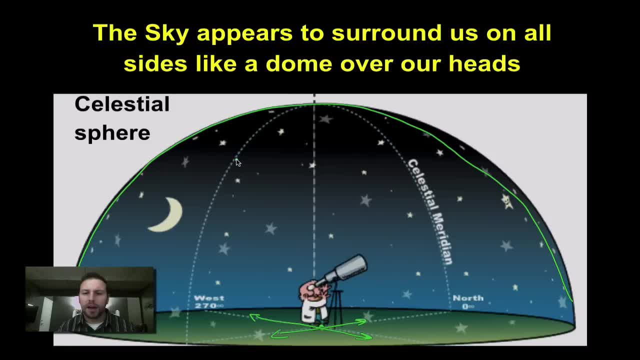 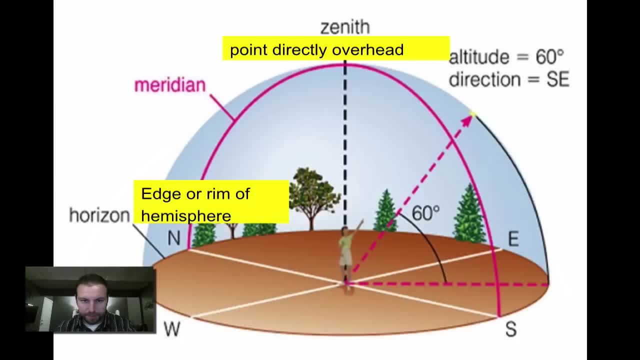 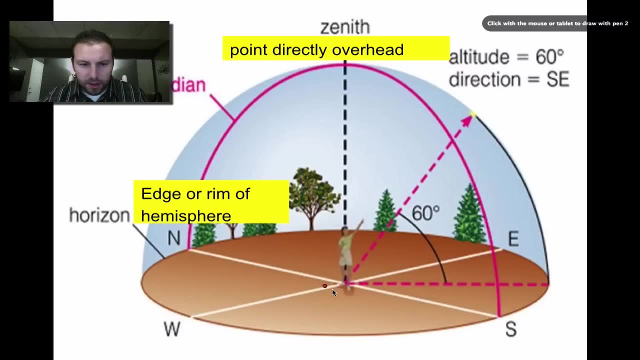 if it's stars, the sun, anything, any other satellites that we see. that's all appearing on the celestial sphere. The celestial sphere has a few parts that we need to take a look at. We have the azimuth direction right around here, on the bottom, Right here, where the dome meets. 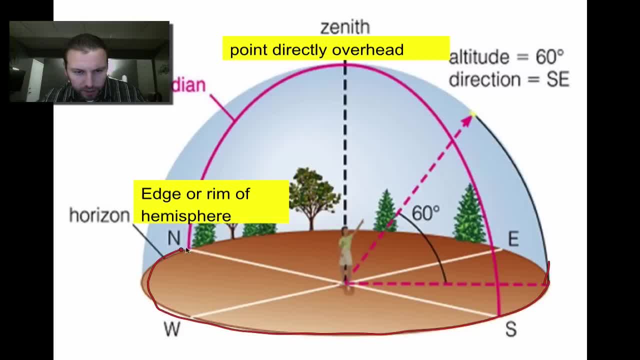 this is our horizon. If you were to go to the beach and look straight out into the water and where the sky meets the land, that's your horizon. The zenith is the point directly above you. so if you look up, that's your zenith. Depending on where you are, really, your zenith is always going to be directly above you. 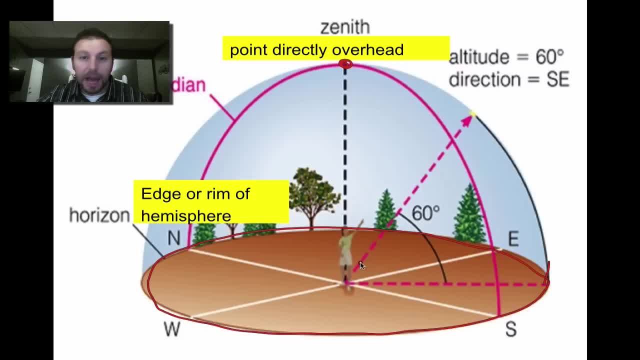 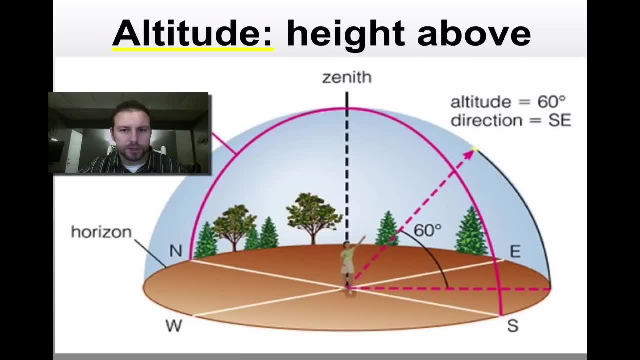 And we also have our altitude right here and azimuth, which we're going to go over next. Our altitude is our height above the horizon, measured in time In degrees. So it's our height above the horizon in degrees. So what does that mean? So our zenith, if we make an angle with the ground. 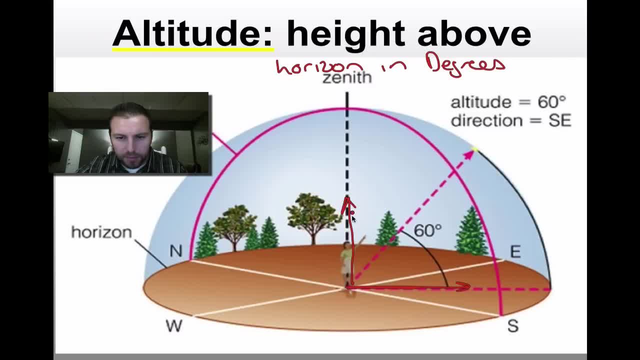 without looking at the horizon and then straight up, we would have a 90-degree angle. Our zenith is always 90 degrees. The horizon is always zero degrees, Anything in between. that is a judgment call You have to figure out. well, is it halfway looking up? 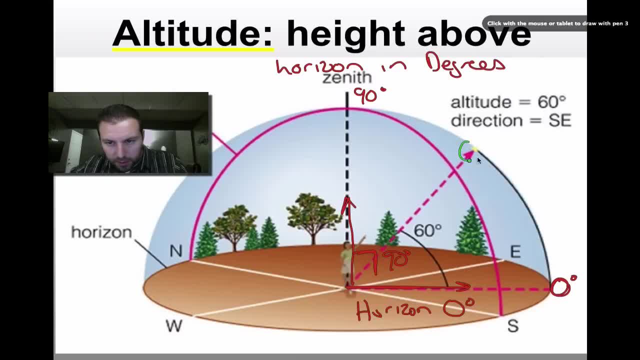 So in this scenario, we're looking at this little star right here, this little yellow spot, And let's clear this to make it look better. If we look at the horizon right here as 0, straight above is 90, then this is somewhere in between. 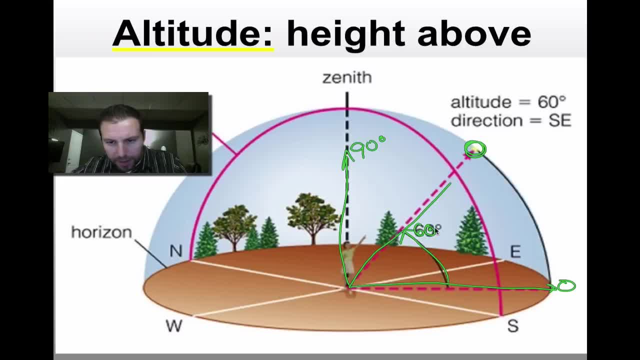 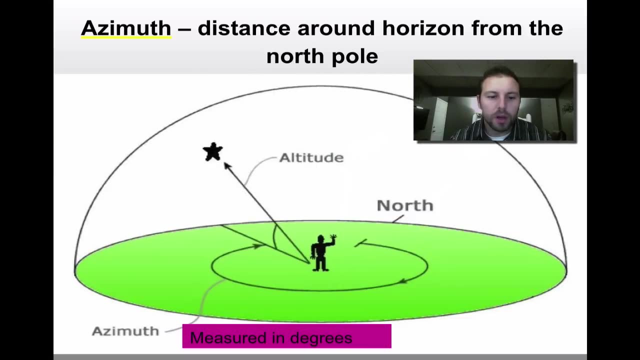 that angle And we're looking at about 60 degrees right here. So your altitude is your height above the horizon in degrees. Then we have our azimuth direction. Our azimuth direction is our distance around the horizon from the north pole, also measured in degrees.